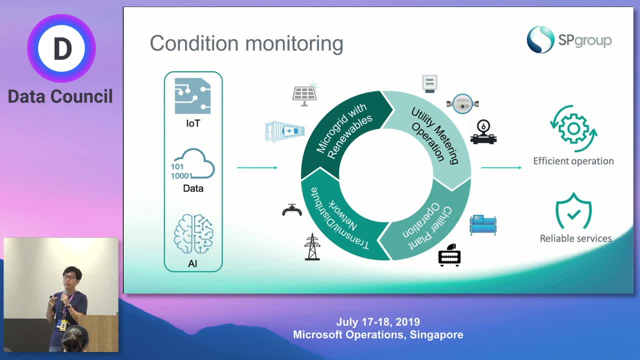 So this is also especially true for the energy and industrial space. So for us, for SP Group, actually, we have a lot of use case which we need, a condition monitoring. So, for example, we need to monitor or check the status of the every single meters in every. 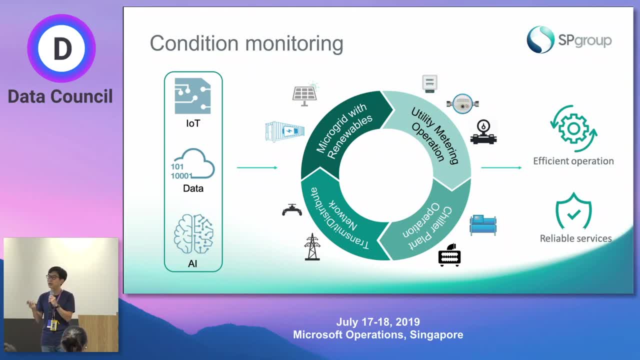 house to make sure our metering and building services is accurate. So for our district cooling business, we need to make sure the cooling tower and chiller is functional properly to provide the cooling supply, for example. So for the micro grid, with new renewables, then we have new things like the solar panel. 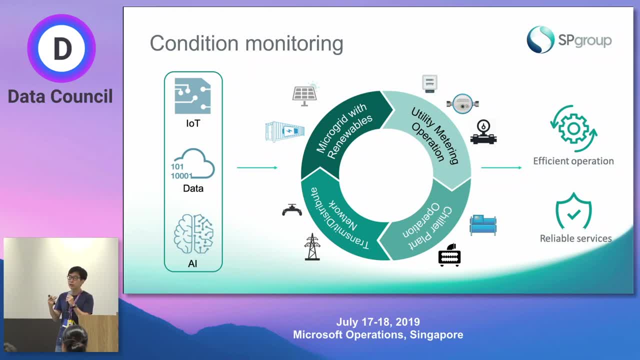 the energy storage system need to function properly to make sure we get the most economic dispatch to supply the energy. And, in terms of core business, the transmission and distribution network. then we have a lot more. More are conditional monitoring use case. We need to monitor the transformer, a lot of equipments inside the network right. 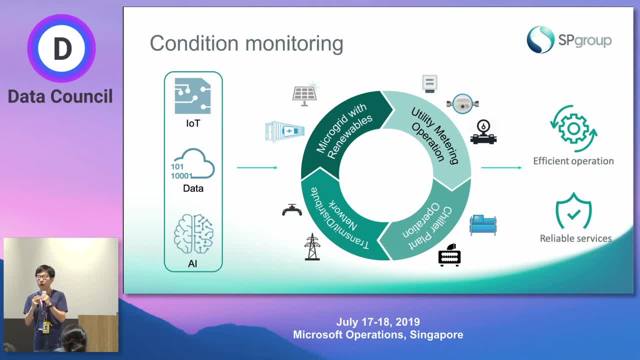 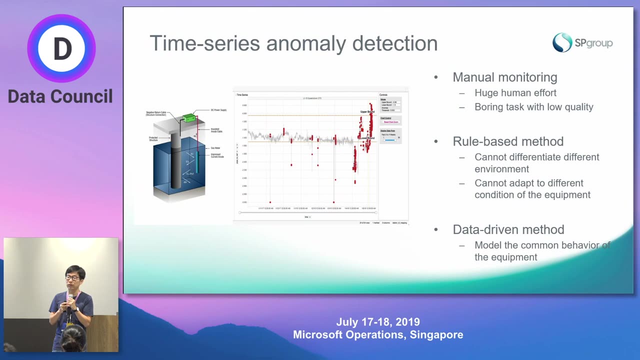 So providing a better condition monitoring will help our business to improve our operation and make sure our services is reliable. So that's the goal we want to achieve, And as one of the important step for the condition monitoring is anomaly detection. So anomaly detection focuses on identifying the data points that do not conform to the 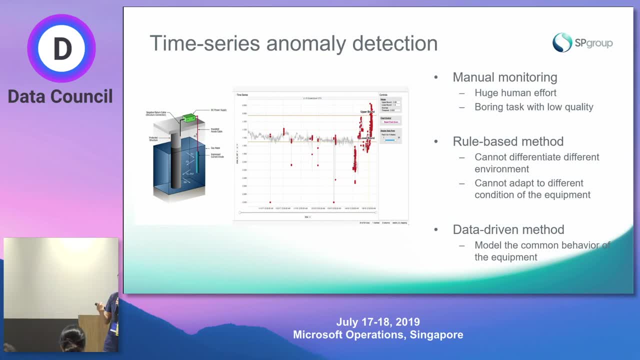 normal, expected behavior of the system or the process. So in general there are three types of the anomaly detection methods. So the manual methods rely on the manual inspection conducted by the human But it requires a lot of human efforts So it cannot be scaled up to handle a large volume or large number of the data. 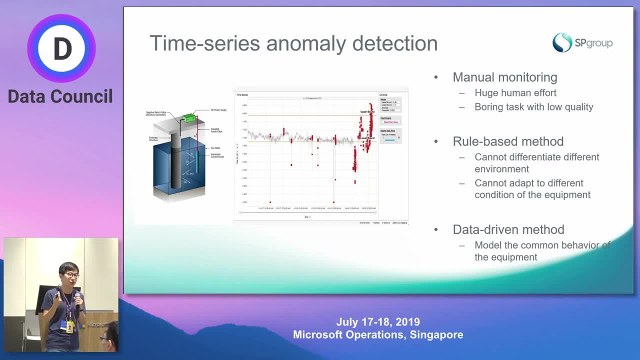 And second, this kind of inspection work is tedious and boring. So the inspection quality- It's not The quality normally- will degrade after the first initial period. So the staff may be very happy to do the inspection for the first half first month. 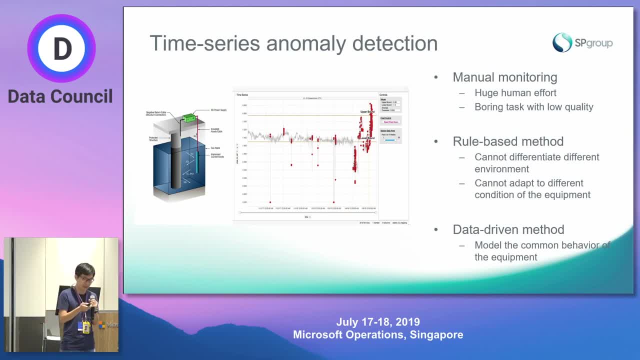 But after that I think it's not sustainable. right, And second type of method is the rule base. So in general, the rule base work like: you will set up the minimum and maximum value for the measurement according to the OEM spec, So anything within the range is deemed as a normal. 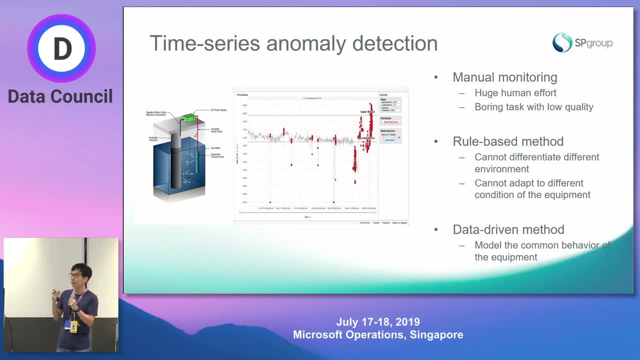 Anything outside of the range is deemed as abnormal. But the disadvantage of the rule base method is: first, these methods introduce a lot of false alarm. Second, this fixed setup is not adapt to the different environment, different situation. So just imagine the same type of equipment of the same brand when they deploy into different 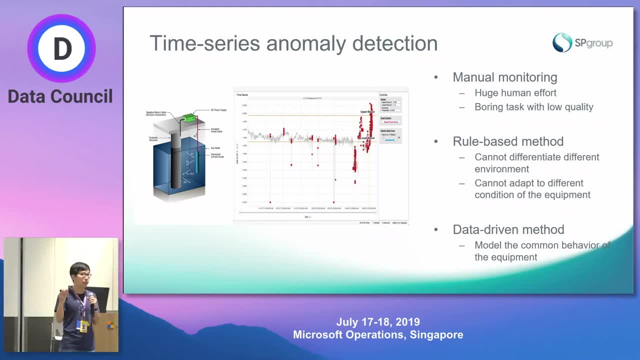 environment and the working condition is different. So with time evolve the behavior of the equipment will be different. So some behavior In one situation is a normal behavior, but if you shift to another environment the meaning is different, It is become abnormal. 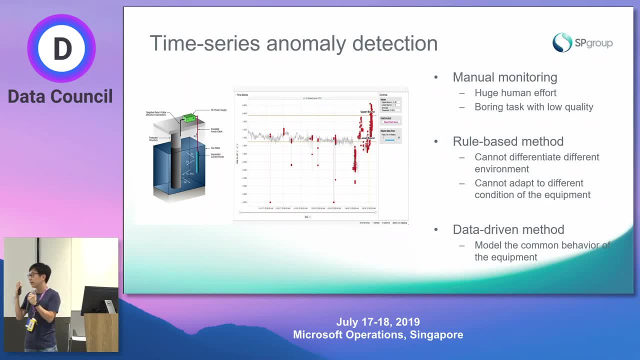 So the rule cannot capture these kind of things. So that's why the third category, data-driven methods, is preferred. So, instead of relying on human inspection or rules, these kind of methods will lend the common behavior of the equipment from the data and detect anything different from. 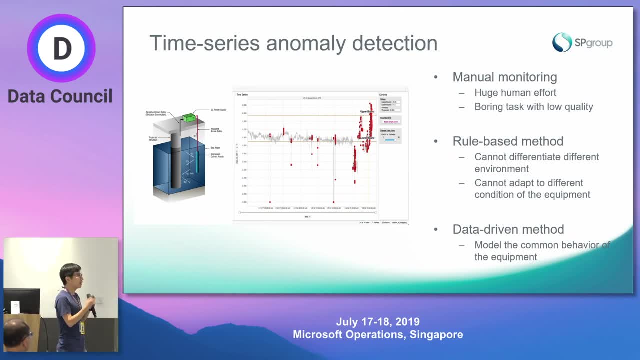 the common behavior as the anomaly. But The adoption of these data-driven methods for anomaly detection is hard actually, Because in a very- I mean very often- situation, if you ask the users they will say: okay, I like this sound mess. 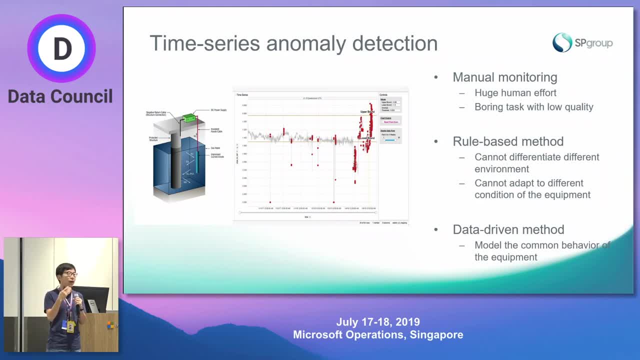 I want the anomaly detection, But when you go into the detail you ask: what are the, what are the anomaly you try to detect? Then they will tell you: I don't know. I don't know what kind of overview I'm looking for. 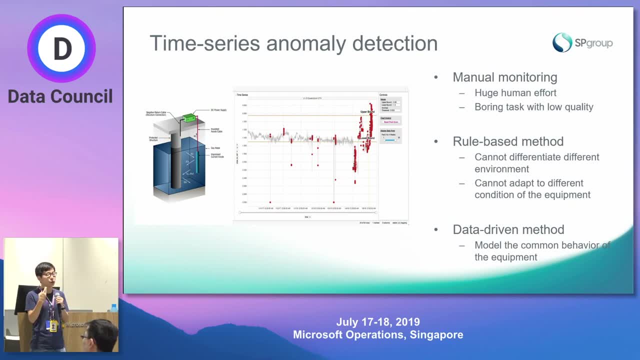 Then what kind of business value you are attracting there. So our solution to this: actually we want to provide a low cost, easy to use, out of box solution To the users. We want them to explore as much as possible the use case. 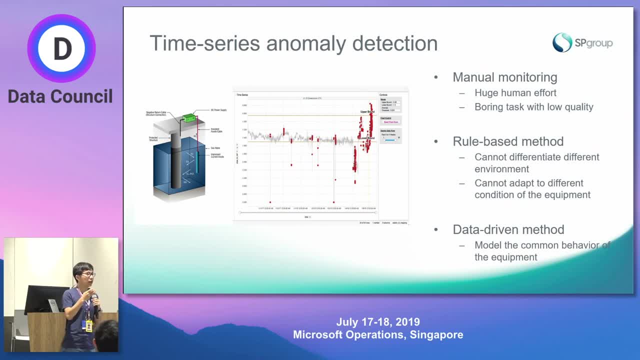 As the first stage. Then they will give the feedback about some of the low value use case. They can directly use the out of box solution For some other use case. if you need a very accurate- I mean more advanced- solutions, then you go into a customization mode. 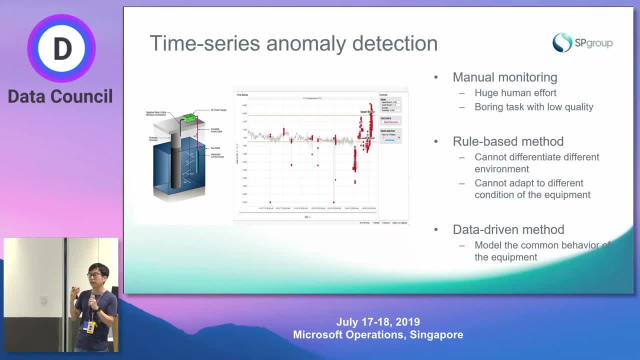 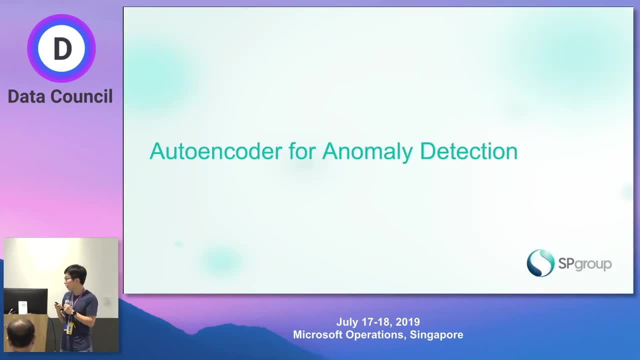 So today, what I'm going to show is is that our effort to try to make a low cost, easy to use, out of box solution for anomaly detection. So auto encoder is one of the common methods being used for anomaly detection. So I may want to ask the question: how many of you know the auto encoder? 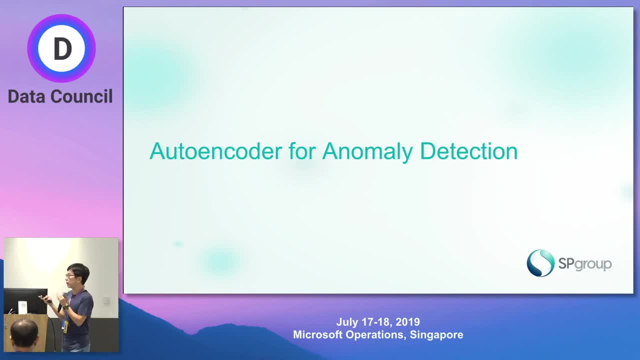 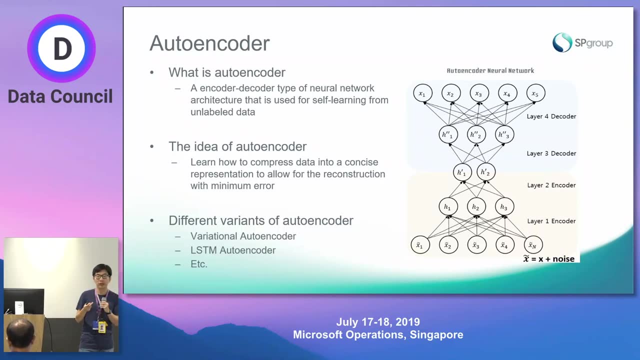 Okay, So a few of them, So I will give a very quick introduction. So auto encoder is the type of neural network with the encoder and decoder architecture. So the idea of the auto encoder, it is kind of self-learning. Self-learning means that the unlabeled data is used. the data itself is used as a label. 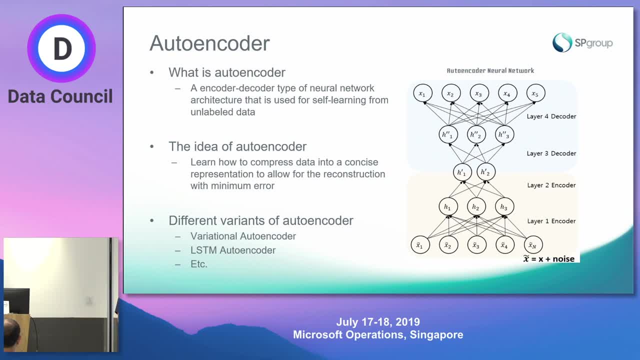 to train the network to learn how to reconstruct the signals. So the output of the network is target to be as similar as possible to the input data. So the idea behind the auto encoder: normally they will introduce information bottleneck. for the encoder part It means you want to learn a concise representation of the input data. 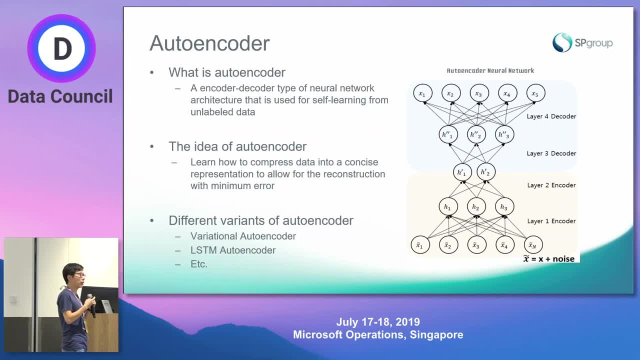 And then the decoder will. then how can I reconstruct the original signals from the concise representation to make it as similar as to the input data? There are quite a lot of different variants of the standard auto encoder. So, for example, the variational auto encoder will try to encode the input data to the parameter. 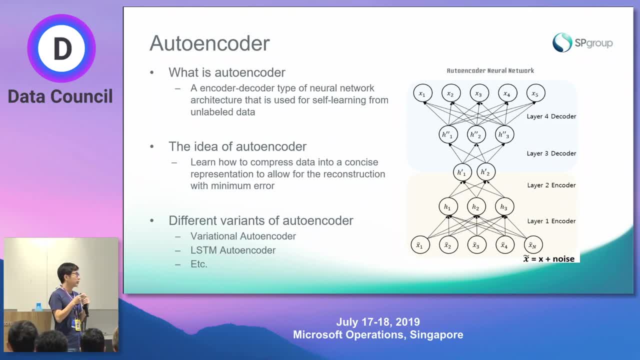 of the data distribution instead of the data itself, Because it will allow you to do the sampling out of this distribution to generate the new samples And for time series, the LSTM auto encoder will replace the MLP with the LSTM to try to then automatically learn the feature which can better represent the time series. 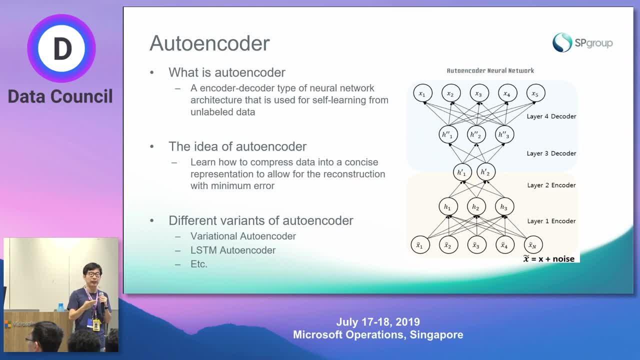 So the method we are talking about later actually is independent about what kind of auto encoder you use. You can apply different variants of the auto encoder, But for the talk I will use the most standard MLP auto encoder And this is the general framework. 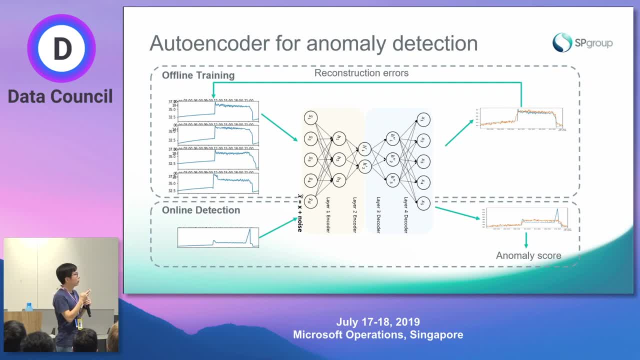 How to apply the auto encoder for an orbit detection. So during the training phase you are given a collection of a subsequent windows. By encoding and decoding these subsequent windows you get the reconstruction error. So the error will be back propagate through the network. to update the network, allow it. 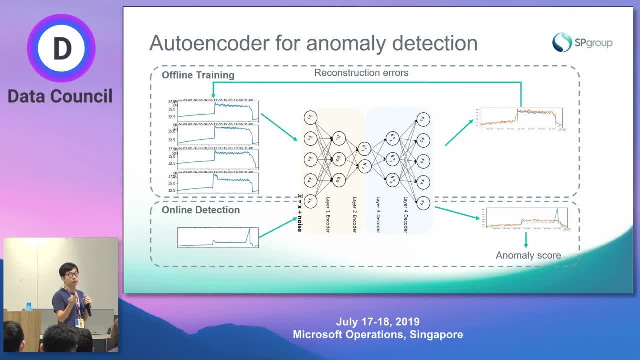 to learn to minimize the reconstruction error from the input to output And then, after the model is trained for online detection, A new subsequent window will pass through the network, encoded and decoded. Then you can compute the reconstruction error from that. So if the new inputs of subsequent windows, the essential information, is different from 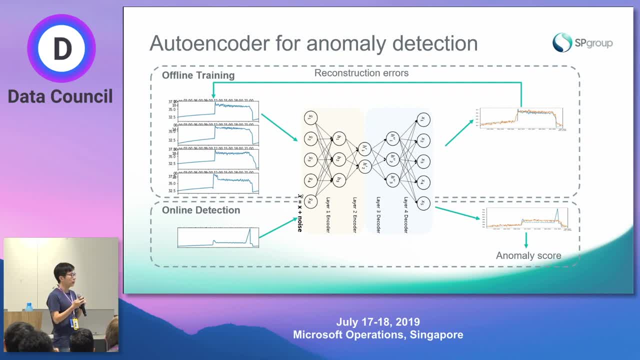 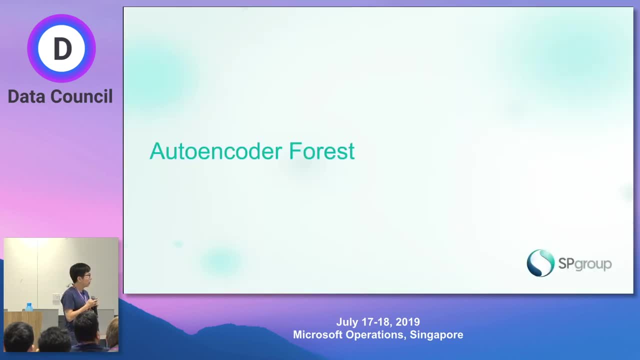 the training data, then your model cannot be reconstructed, So you will get a high reconstruction error, And that's how the anomaly was detected. So now I want to go to The core part about how the new methods we call the auto encoder forest is designed. 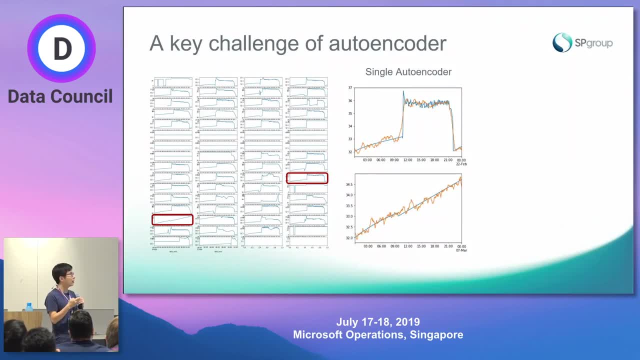 So I will go to the motivation. So the first thing I want to talk about is there's a key challenge if you want to directly apply the auto encoder. So this is one IoT time series example. I highlight two windows. One is the common daily profile. 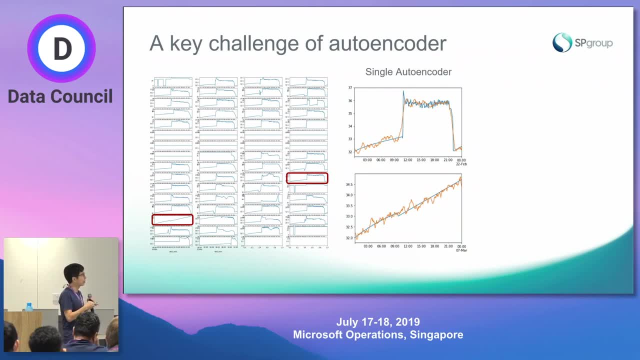 Another one is actually an outlier. It's a special event. So this is the common daily profile. So this is the common daily profile. So this is the common daily profile for this cooling tower system. This is the special event. At that day, the cooling tower, the fan, is not turned on. 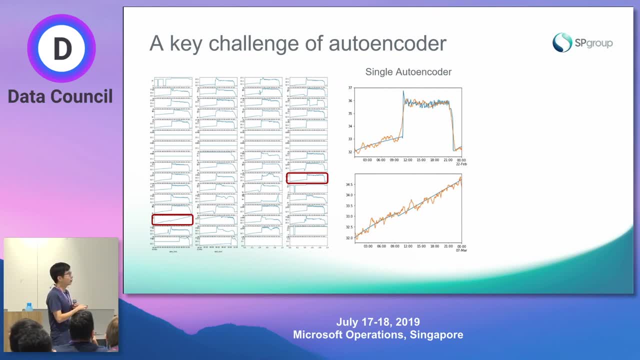 But if you directly apply the auto encoder, you train a single auto encoder from the whole data set. you can see, actually the auto encoder can encode both of the profile quite well. This is not the expected result we want to see. We want to see you can differentiate. 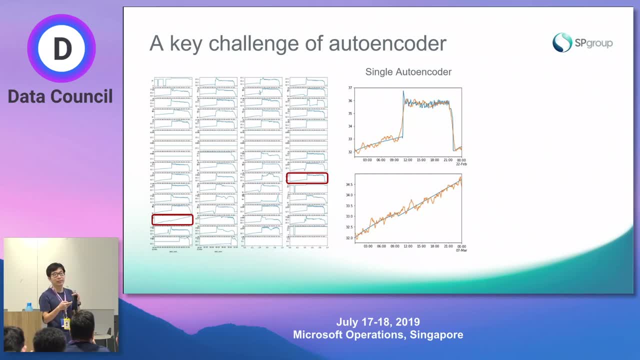 So the reason is the auto encoder. The auto encoder is kind of self-learning, So there's no easy way for it to do something like a cross rotation to see how good or how bad the train model is. So it probably can encode everything. 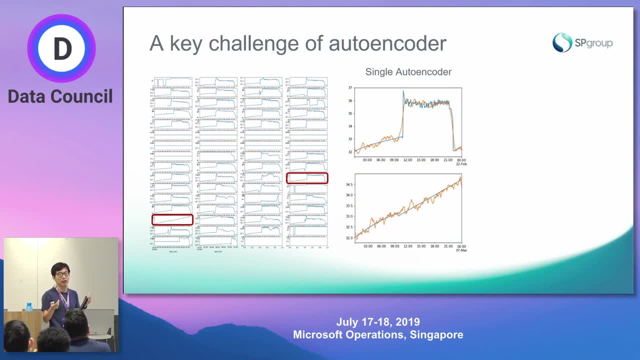 It can encode whatever data it passed through to you. It basically can encode everything. Then you cannot differentiate the normal thing and the normal things. But even you are given, let's say, another scenario, you are given historical anomaly examples, It still faces these issues because the whole training data set has a lot of varieties. 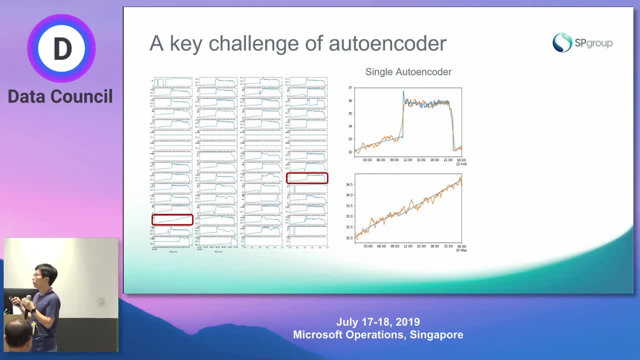 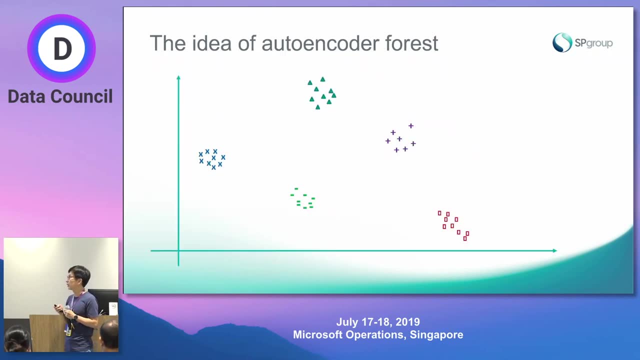 So if you train a single model on that, the model must be able to cover all the variety inside your data. So I will use a synthesized example to illustrate this. So suppose this is the data set you are given And one project to 2D space is something like this: 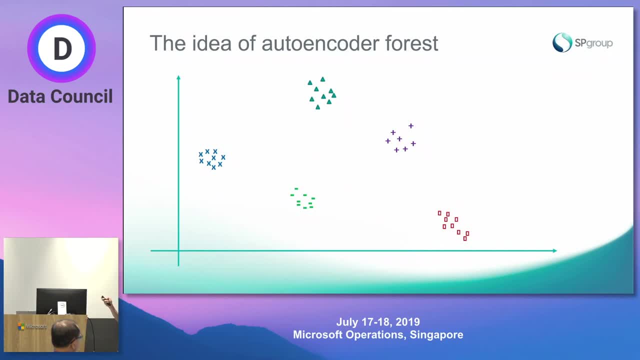 So you can see there are multiple structures inside your time series. So when you use a single auto encoder to model this, it basically will cover the whole space, cover every single structure. Then there's understanding. Unnecessarily you cannot avoid some area outside of the data. 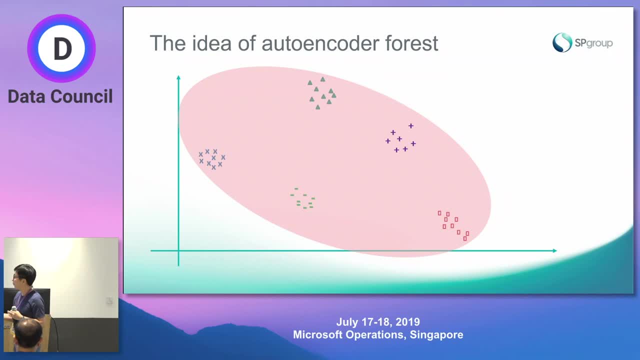 So you unnecessarily involve the area, like, for example, in the middle. This is the data, This is the area outside of the data and where the unseen anomaly may appear in here in future. So the idea may be very simple, right? So instead of building one auto encoder, actual thinking is that, how about I build multiple? 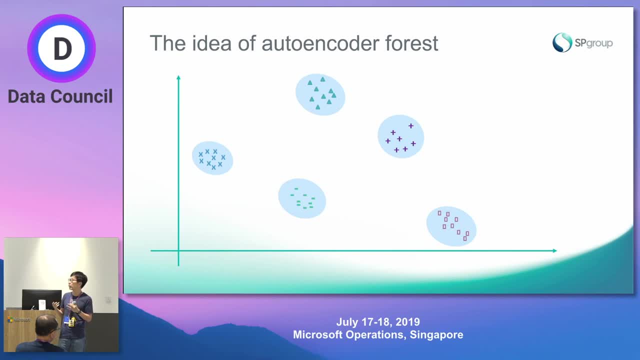 models. One focus on individual models. One focus on individual structure of the cluster And by doing this you now you only try your best to every single model- will really focus on the specific pattern that the training data pass through it And you will try to avoid as much as possible the unnecessary area you try to involve. 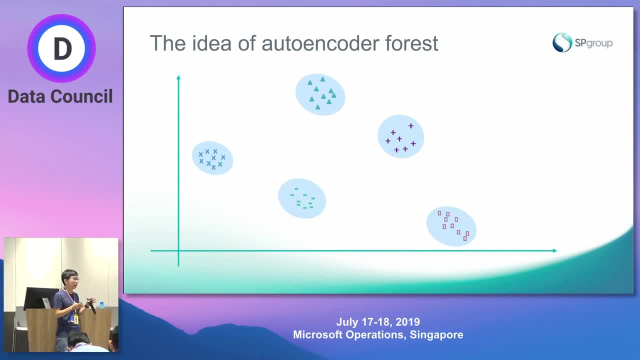 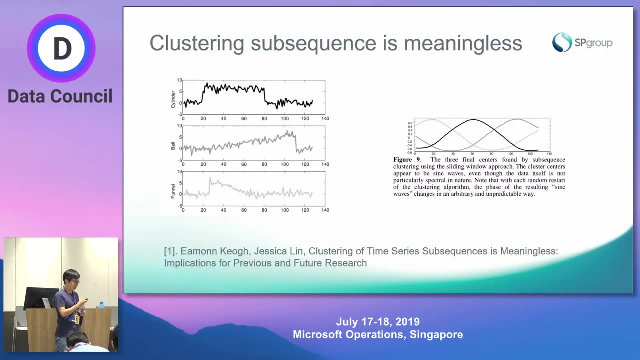 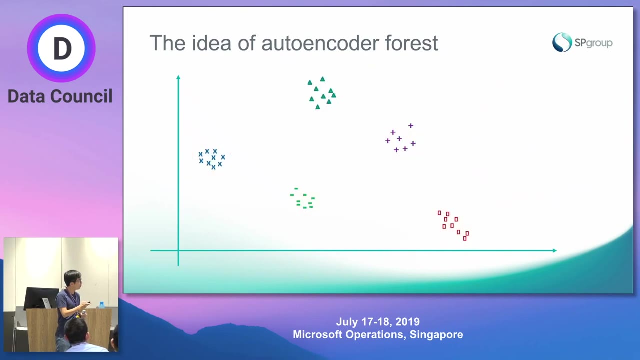 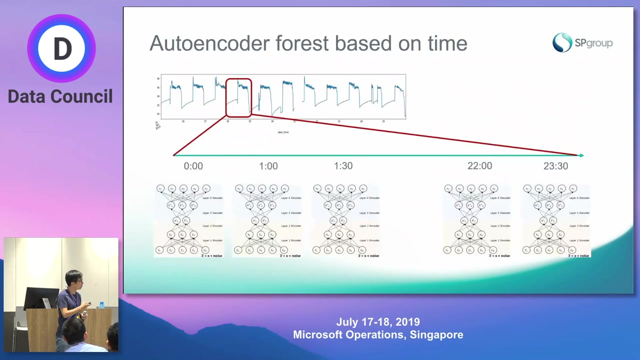 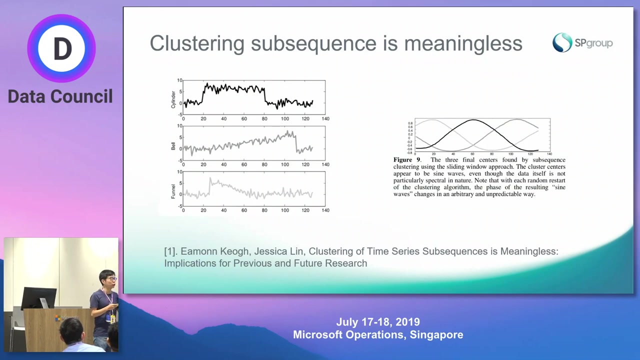 So this is the motivation about the challenge and the basic idea underlying the auto encoder forest: We try to do the problem. So if you are So let's continue. So the nature idea is like how? Now the question is: how do you identify the different cluster inside your data? 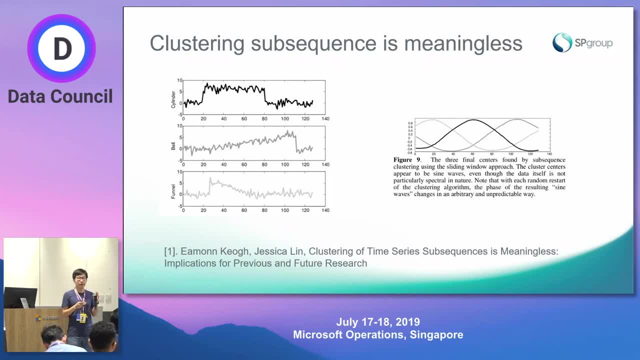 Then you can train the individual auto encoder. So from the previous illustration you may think the most intuitive way is that If you are the person learning the data, you can learn that by applying the clustering on the data. Then for each detected cluster, I will try to learn auto encoder from that. 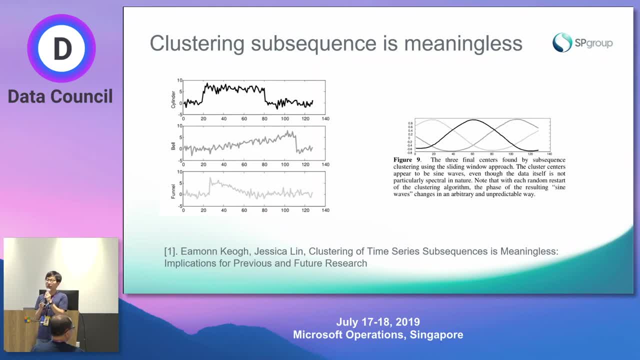 But it won't work. Actually, it will fail if you try the clustering on the subsequence, Because the Eamon and Jessica has studied this problem in their paper, So they found an interesting phenomenon about the clustering: the subsequence is meaningless. Their conclusion is that no matter what kind of the time-series data is, if you apply the 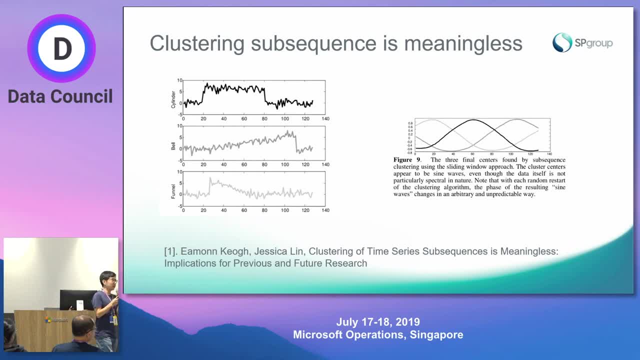 apply the clustering on the subsequence, the detected cluster center will be something I show in the right figure. It's something similar to the sine wave. So it means if you apply the clustering on that based on subsequence, the cluster you get actually the variety. 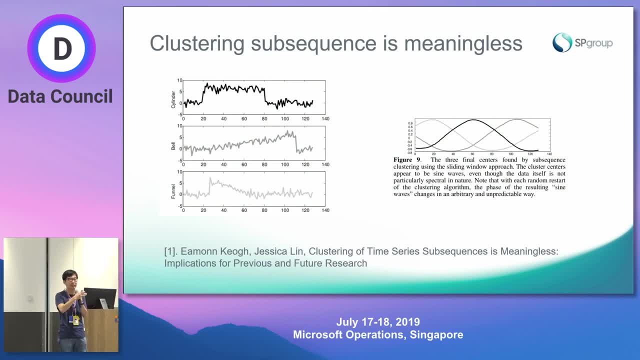 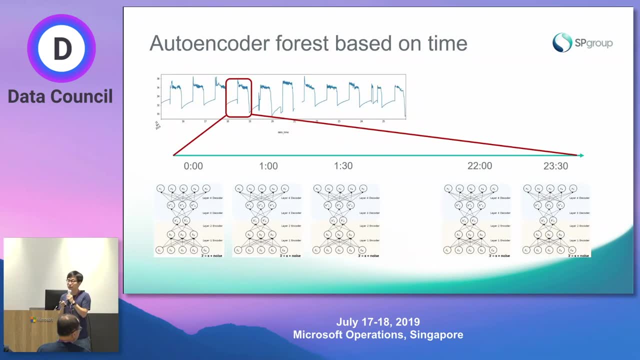 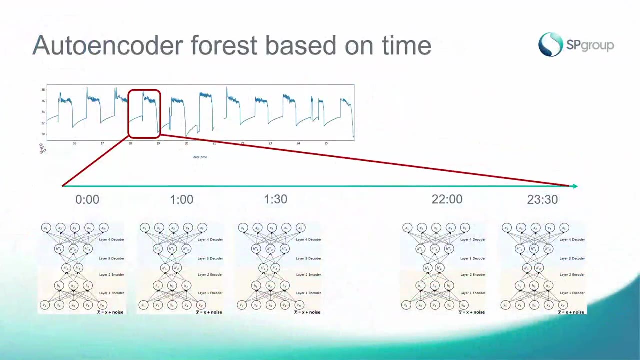 of the data didn't reduce. It still remained the same because it covered the whole spectrum of the sequence. Then the question is, if the clustering doesn't work, then what kind of information we can rely on to get the different group from the data. So what we try to explore 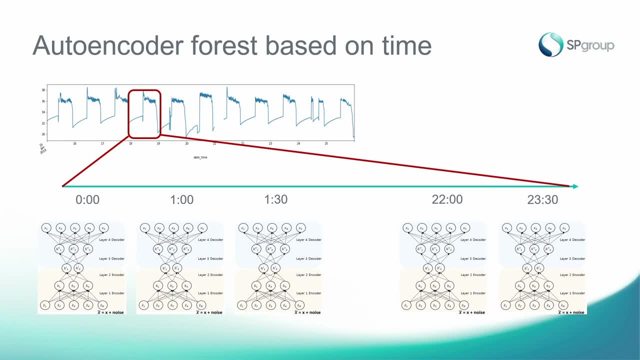 is the time information which is naturally available in any kind of time series. So this is an example. So, given the time series, if you can be able to detect the repeating period from the time series, For example, let's say this is the time series, Its pattern repeats every day. Then according to how many points? 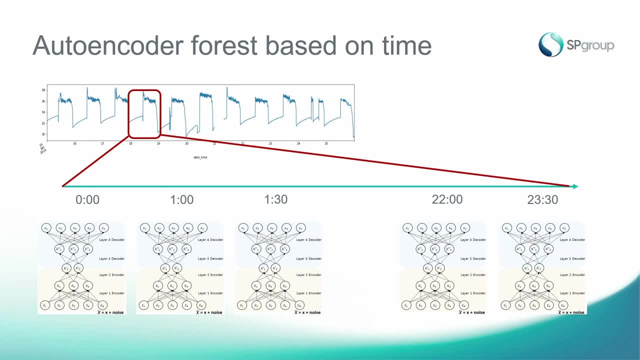 you sample within a period, within a day, you can align all the subwindows sampling at the same time. So, for example, if it's a daily pattern, it samples every hour, right? So 5 o'clock, 5 am in the morning, If you collect all the subsequence windows aligned. 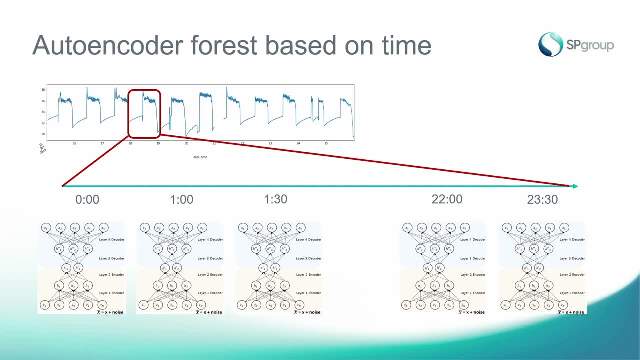 on the 5 am across the last three months. this is naturally a cluster because it shows you the similar subsequence patterns from the data. So by doing this we actually avoid a not working solution. to apply the clustering, We naturally use the available information about the time. 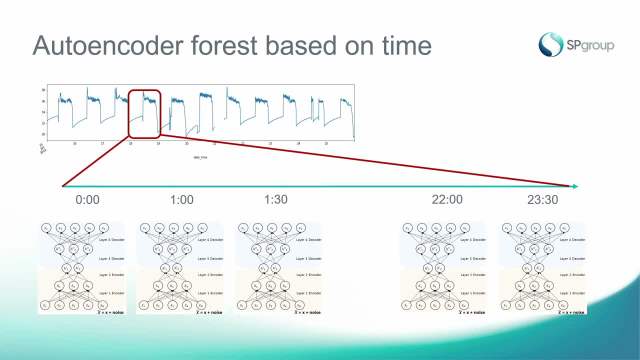 in the time series. But I just want to highlight, our alignment is not directly based on the timestamp. So just now I highlighted an example of the daily profile, but the period could be anything. For example, your period could be three hours. Then your actual timestamp. 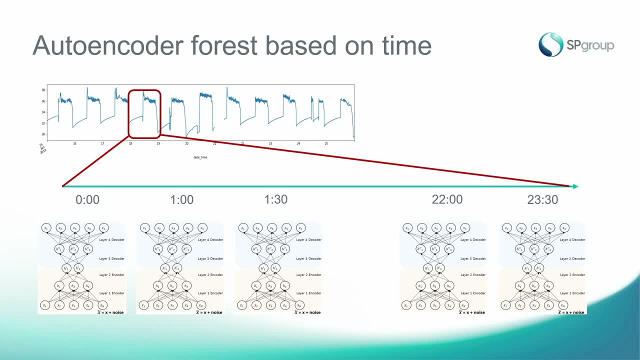 is not exactly the same. So you can see that the time stamp is not exactly the same. So you basically need to say: you need to put the index on your sampling data And, let's say, the first sampling point of every period. this is my first cluster. 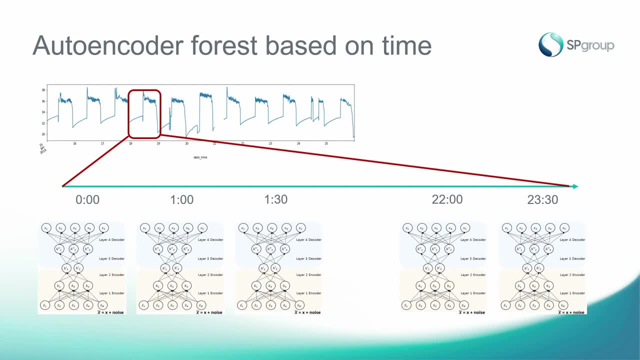 The second sampling point of all the periods in my training data. this is a second cluster I will get. So is it clear? I hope it's clear. So this is a core part of our methods. so Auto-Encoder Forest. Once you know this group, then the idea is rather simple For each group. 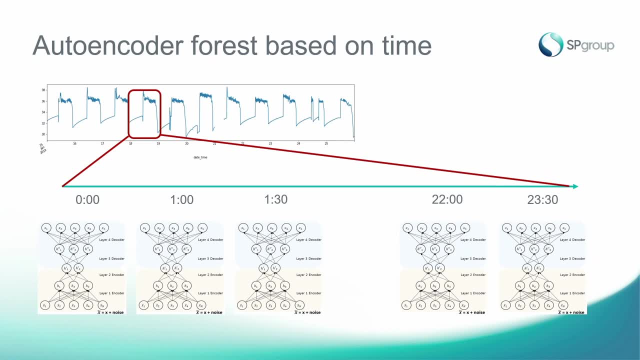 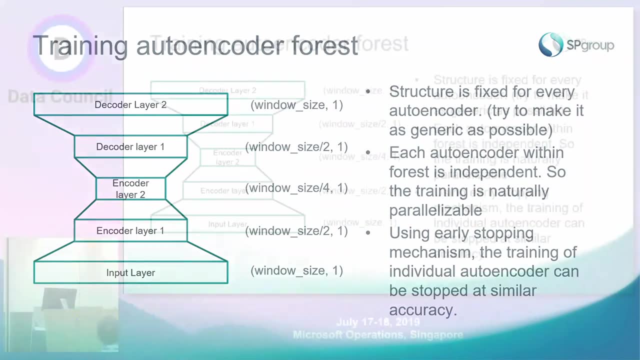 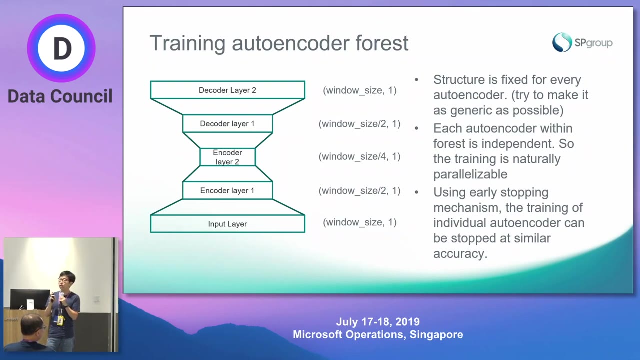 then you train a single data sequence. So every day, every minute, once a new你的 an individual autoencoder based on this subgroup of the data only. I want to talk a little bit about the actual training of the autoencoder. So we didn't spend a lot of effort on fine-tuning the architecture of the autoencoder. 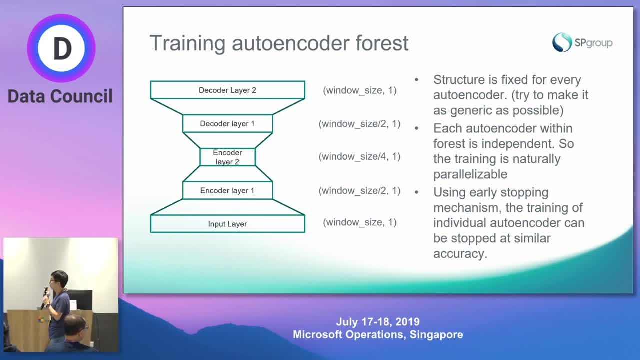 So instead we fixed the structure like autoencoder has two layers of encoder, Each one tries to reduce the input dimension to half And we have two layers of decoder, Each one tries to increase the input dimension to two times. So the activate function: we all use the RERU, except the last layer. we use the linear activation. 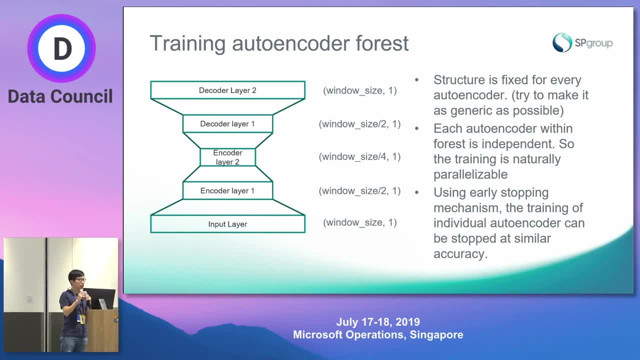 function. So the idea to use the standard structure and the standard training process. we use the early stop mechanism to stop the training if the benchmark performance is reached. Otherwise we run the maximum number of epochs before the training And the training is complete. 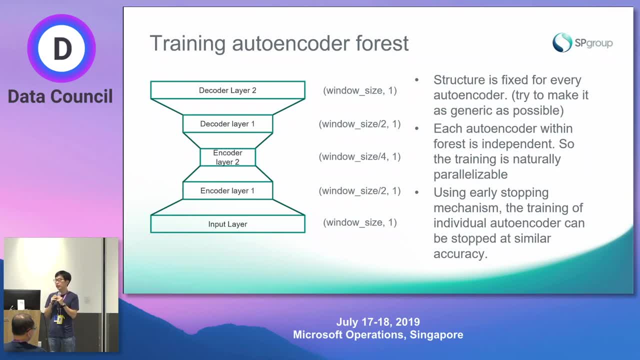 So what we want to try to achieve is that we want to use this standardized architecture and training process to train on every single individual autoencoder across different type of the IoT stream, to reduce the cost, to avoid unnecessary customization. That's how we want to achieve like: lower down the cost of the solution, push the adoption. 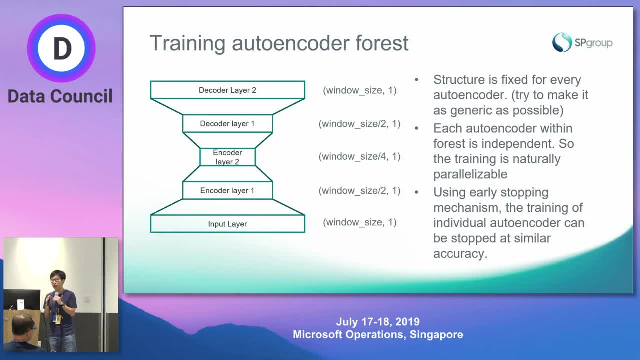 for this And actually we found it works quite well across different type of the autoencoder. The reason why we want to achieve this is because we want to reduce the cost of the automation. The reason I probably can explain is because now the training data for every single autoencoder. 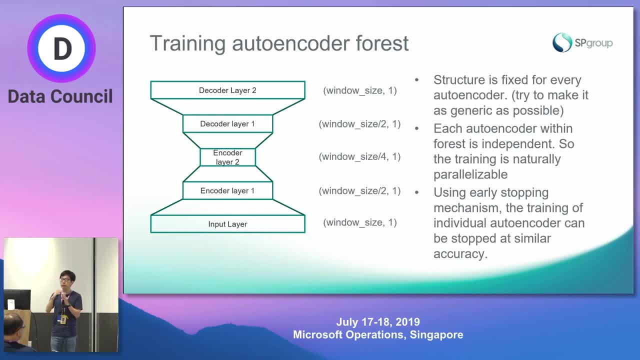 is very focused, Because I only pass the subgroup which you only have, one or two at least, a lot more less than the whole data set to the autoencoder. You really can focus on this pattern only, And this is the result I want to demonstrate. 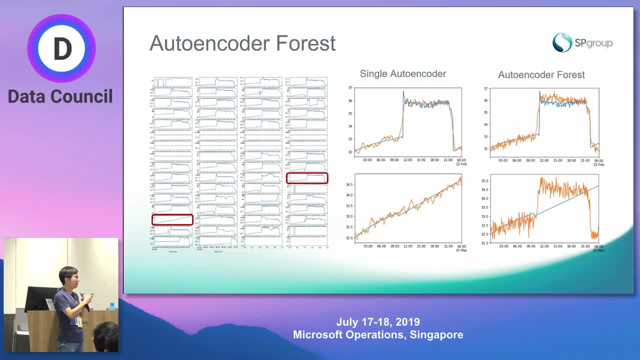 So previously we show for the two patterns, which are very different. single autoencoder actually can encode them. But if you apply the autoencoder forest to that now you can see it can differentiate the two profiles. For the normal profile the autoencoder will encode it quite well. 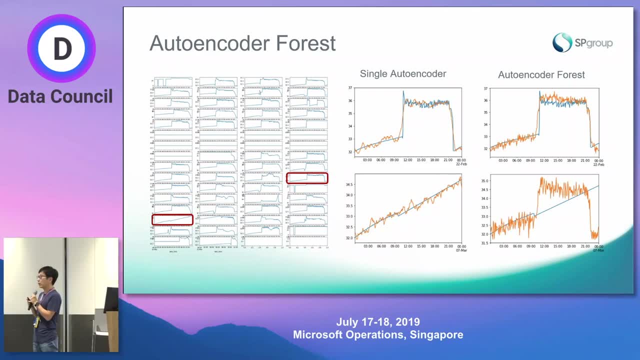 For the unusual profile the autoencoder now cannot reconstruct the signal very well. But I want to highlight actually for the autoencoder forest, even though we have multiple models- in this case the two windows- Actually It is encoded by the same autoencoder because they are aligned at the same time. 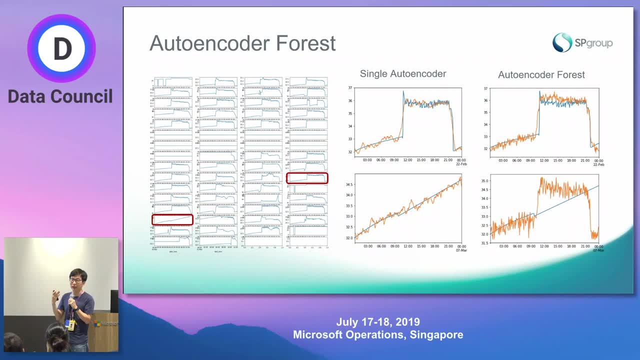 So it's not because now I use a different encoder to encode it and they can differentiate. It's still using the same single autoencoder, but this time this encoder only trained with a specific pattern. You won't be confused by you. give them a lot more pattern to learn. 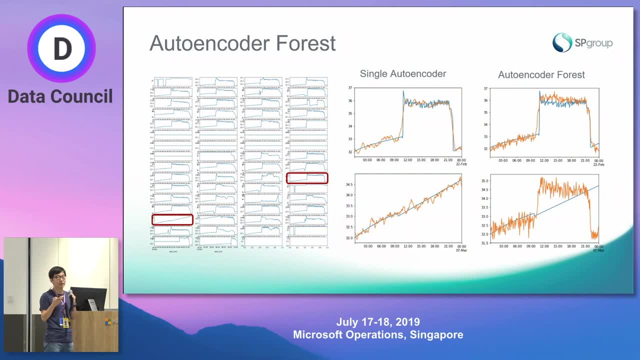 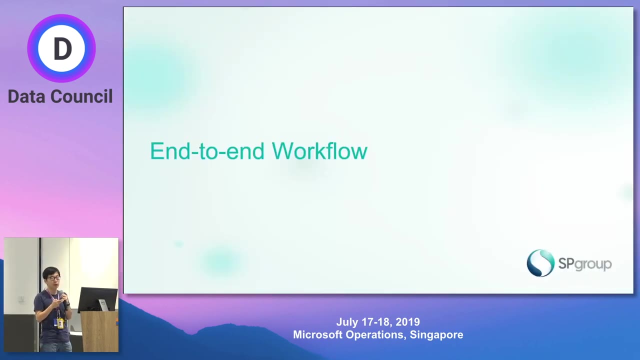 So this is the example I hope I can Illustrate to the audience to make you understand what is the motivation and how we design it and what's the impact and effect. this solution apply when you apply on the real situation. So next I want to talk a bit about the end-to-end workflow. 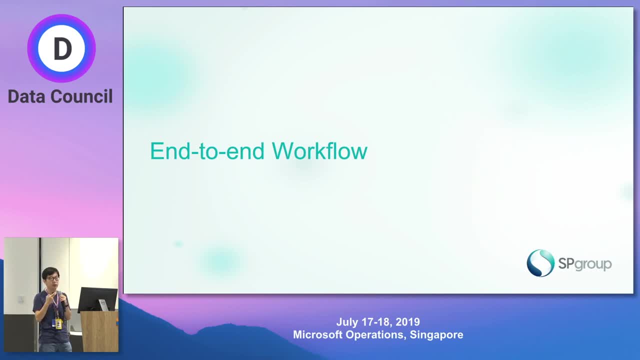 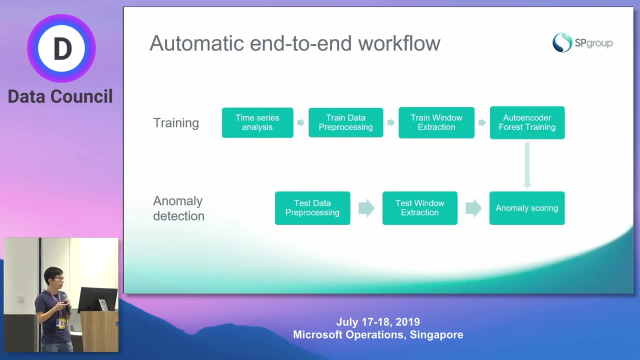 So once you've had a solution to really try this solution, we need to automate it. We need to make it as a service. So this is the standard end-to-end workflow For training. the time series data will go through. We need to apply some time series analysis and processing. 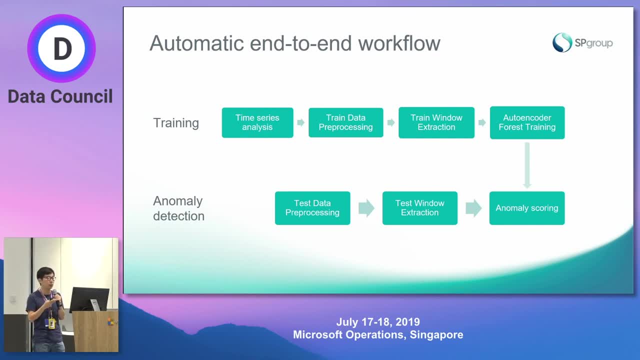 After these two steps, the rolling window at every data point will be extracted as the training data. From there we train the autoencoder forest, which is basically a collection of the autoencoders, And this will complete the training phase. And for the anomaly detection flow, the new test data will be passed through similar processing. 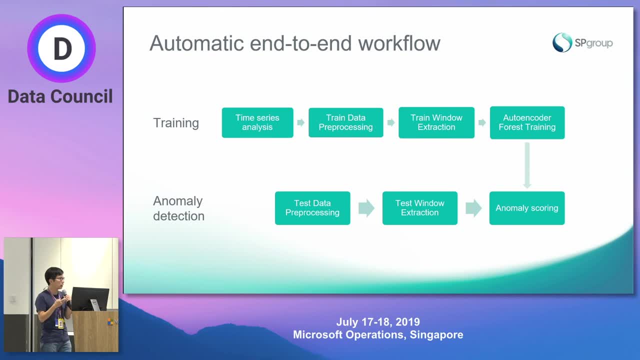 and analysis will be applied on the test data And the rolling window of every single point will be checked and will be sent to the autoencoder. A specific autoencoder will be picked up and score the sequence And this is how you can get the anomaly score. 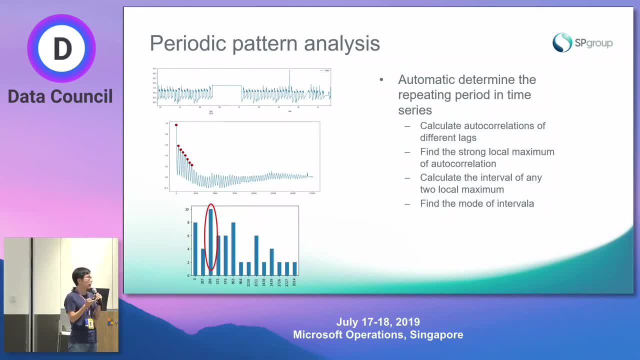 And there are some very important analysis part I want to highlight. First, it's about the periodic pattern analysis, Because we need this period to determine every data point which cluster it belongs to. So the idea behind is we will compute the local maximum of the autocorrelation. 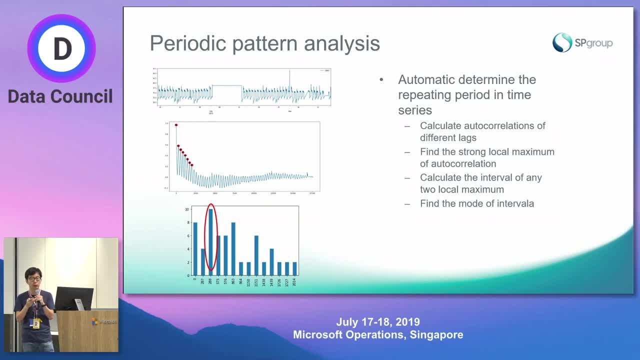 And we will get the mode of the interval between any two local maximum points And you can see from this example. it's a time series data with every five minutes sampling points. It shows the daily patterns, even though there are a lot of deviation. 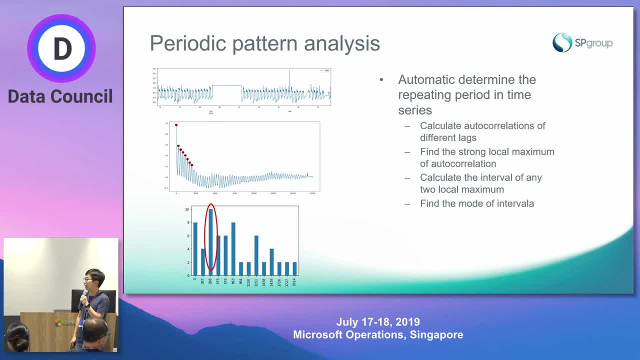 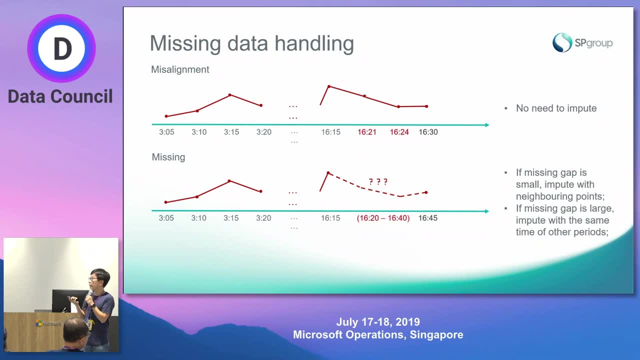 But even in this case, the proposed method will still be able to detect correctly the daily pattern. That's the period. Another important processing I want to highlight is about the missing data handling. So for the IoT time series, there are specific things about misalignment. 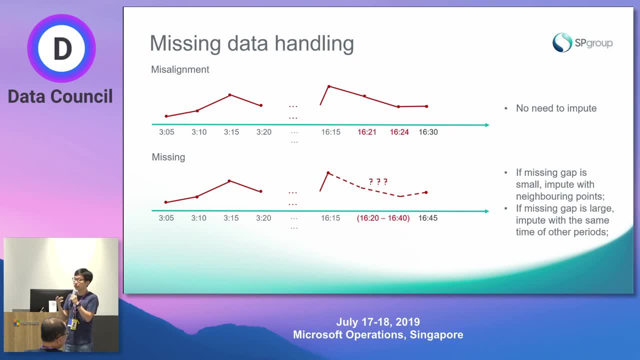 Because you know, the sensor sending the data, due to the sensor issues and network issues, sometimes the interval, even though it's fixed, but the real data sent in, there's a misalignment. So, for example, in the top example the data actually is supposed to come in. 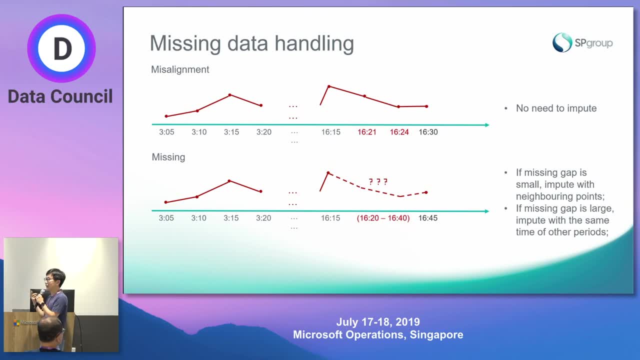 At 4.30,, but the data comes in one minute late. This is what I call a misalignment. In this case, actually, there's no data missing, You just need to align the data points. And in the second case it's like if really there's a big gap, about more than two times. 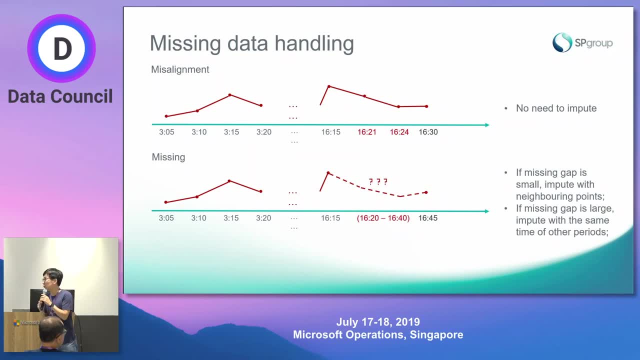 of the interval you don't have, the new data comes in. This is the situation: You have a missing value. So to fill the missing value, we have two strategies. If the gap is very small, we will use the nearby value to fill in the missing data. 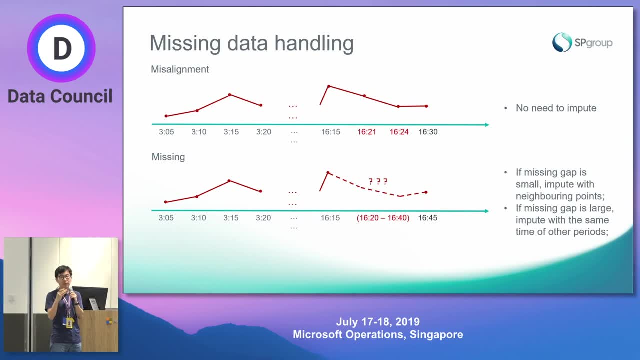 If the gap is very big, then we will use the same period, the median value of the same sampling point from the other period, to fill in the gap, And this is anomaly score. Again, we want to put the anomaly score very simple. 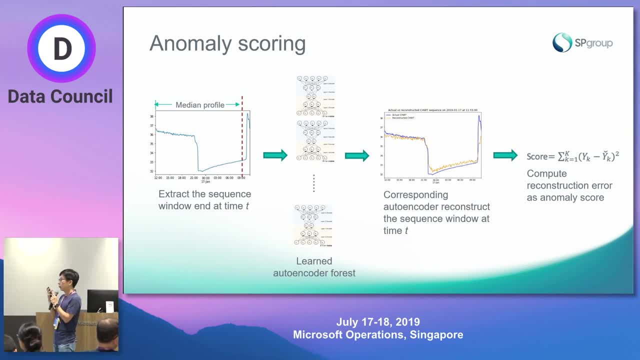 So the idea is that we will get the rolling window from the test data, but we don't want to score the whole windows, So in the first portion we use the median profile to fill in the window And only the last key points are actual value. 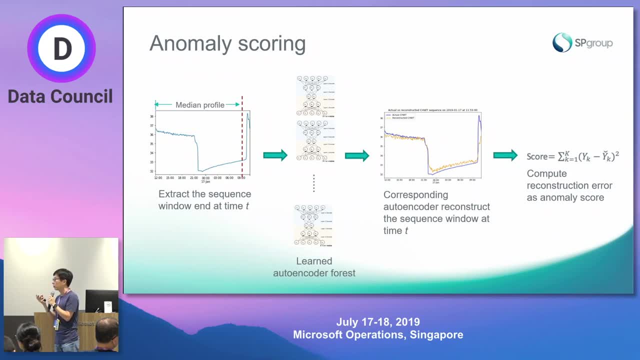 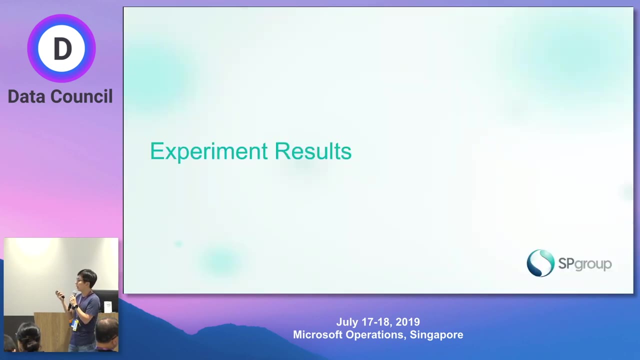 And when this data will pass into the LAN autoencoder forest, a specific autoencoder will be selected and use it to reconstruct the signals. And finally, the Euclidean score was computed between the last key points to compute the reconstruction error. So I will quickly go through a few examples to highlight what is the performance and the 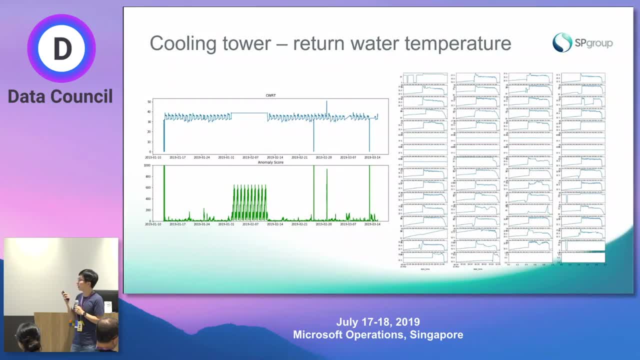 benefit for these methods. So this is the time series data. This is the time series data about cool water return temperature from the cooling tower. So you can see this is a time series, sampling every five minutes And it shows a strong daily pattern, but there's a lot of anomalies. 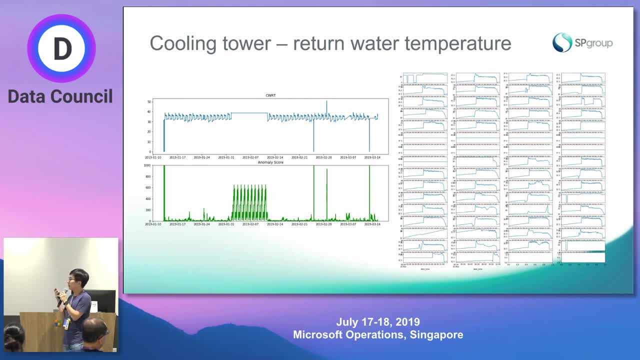 Some anomalies is about the sensor issues. Some anomalies is about the miss operation and some special events. From the left bottom, This is our anomaly score chart So you can see the solution actually successfully detects those very obvious anomalies about the extreme values. You also detect some very subtle anomalies. 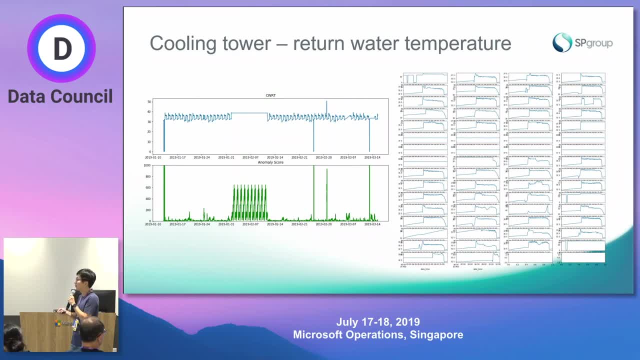 For example, like this part, is a special event corresponding to this anomaly score And also there's a flat line indicating the sensor fault which is highlighted in here. So because our methods assign the real anomaly score for every single data, So it allows the customers actually to progressively select different level of the according to 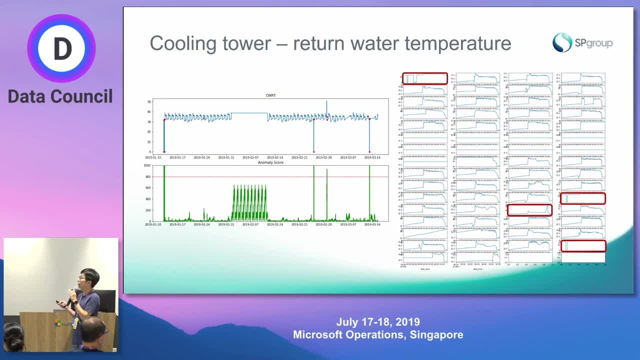 the severity, different level of anomaly to take action. So he can look at the top anomaly score first and then he can go down to a more subtle anomaly score. Then the user actually can find to say what kind of level, what kind of percentage I want. 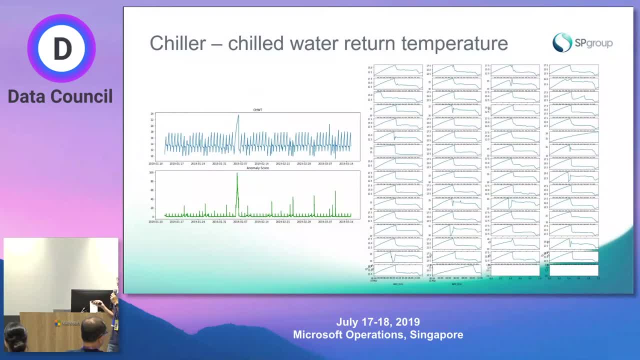 to see in the future about the anomaly. This is another time the IOT time series about the chill water return temperature. So this is the time series. This is the time series. This is the time series. This is the temperature from the chiller. 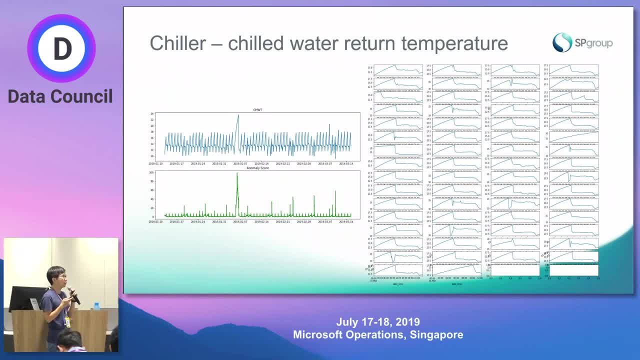 And similarly, this is the time series about the 15 minutes sampling rate And there's a strong sampling irregularity. I mentioned misalignment in this time series But, as I introduced before, our solution can able to handle this kind of irregularity quite. 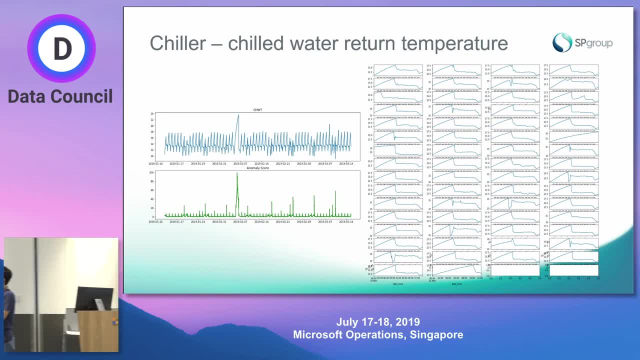 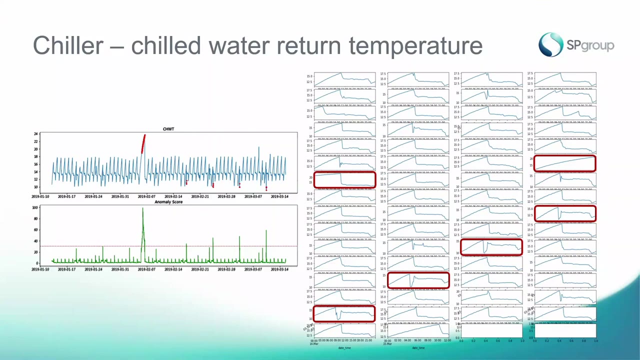 well And you can see it successfully detect the very obvious anomaly here and also detect some kind of misaligned misoperation pattern. So you can see the Besides the top anomaly, the rest of the anomaly is about a single pattern. It's like in the morning the chill water temperature was significant drop and then 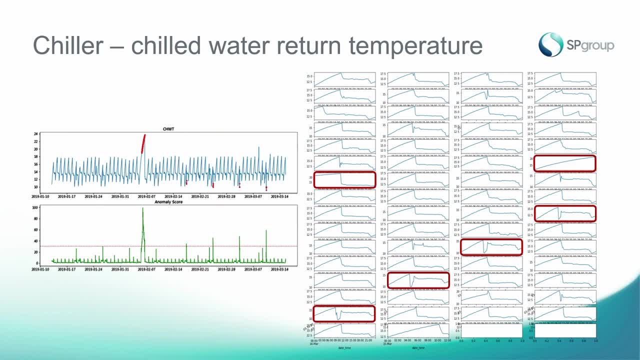 come back. This is something unusual compared to other days, The other days when the temperature go up and then you will immediately go to the normal range, But in these few anomalies you can see the temperature always go up first, go down. very 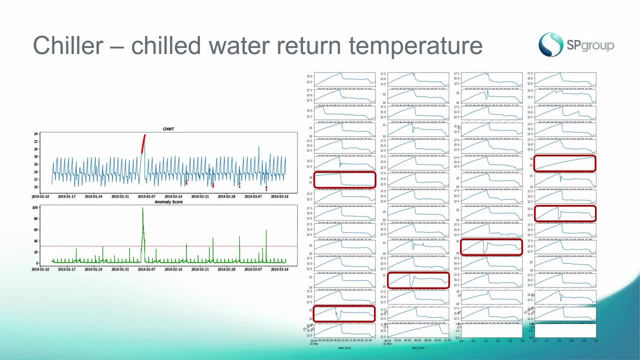 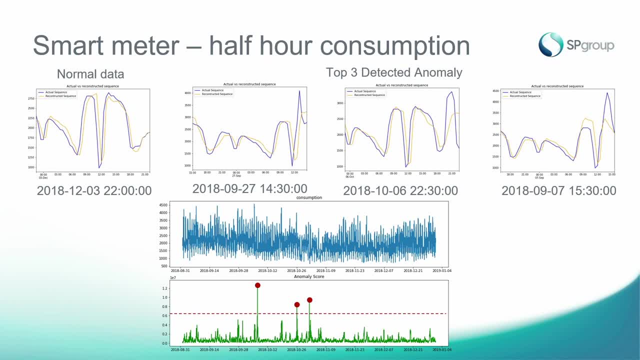 So it's for industrial environment. It's not in your household But similar to a household. it's every half an hour electricity consumption. So from the blue Blue graph you can see this is original sickness. Actually, for human it's not easy to identify. what is the anomaly there? 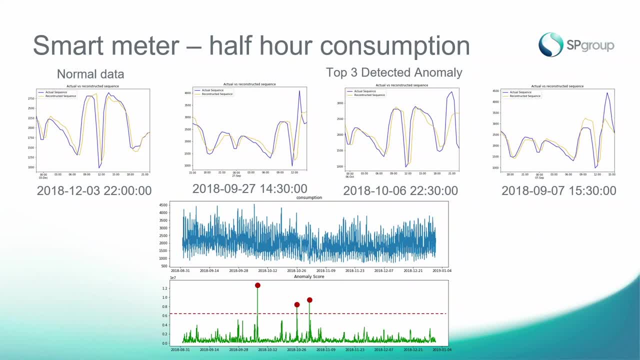 But after our solution applied you can see very clearly a few anomaly pop up with the very high anomaly score. And if you go into the detail about how the autoencoder reconstructs the original signal, actually it provides some explanation why a point was written as a novelty by the model. 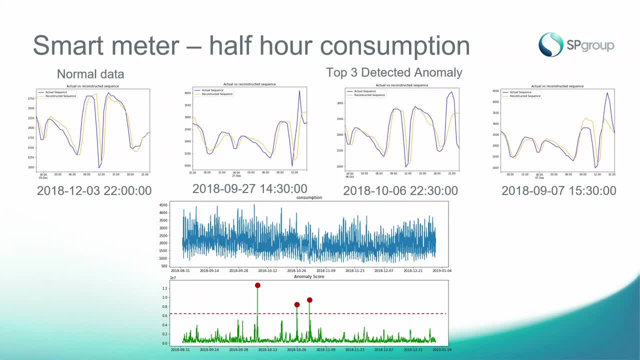 Because, for example, in this day you can see the model actually expects there's no significant jump at the afternoon at 2.30 pm But the input signal, which is deviate from what model believe, has a huge jump consumption around this time. 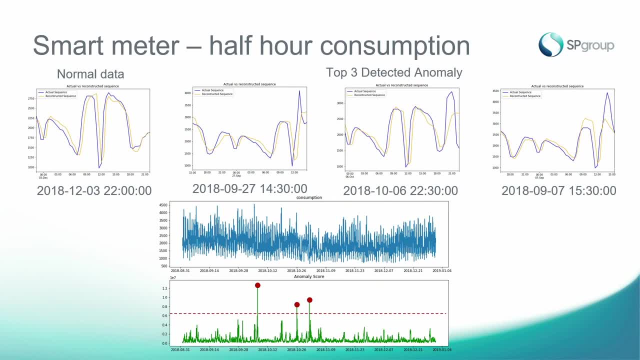 So I think that it's beyond just a black box. The autoencoder, the way how he can reconstruct the input signal, actually provides some information for the staff to understand why there's a novelty, what kind of a novelty happened in this period of time. 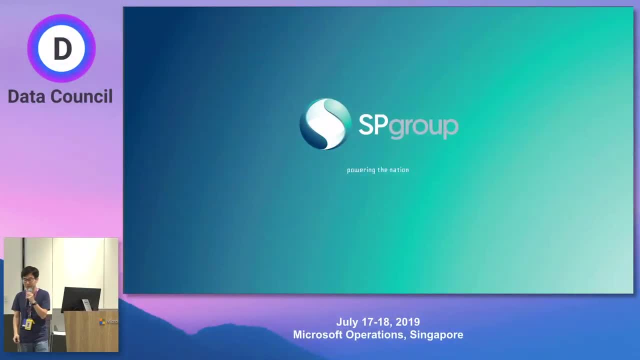 So this is what I want to share. That's all, Thank you, Thank you.